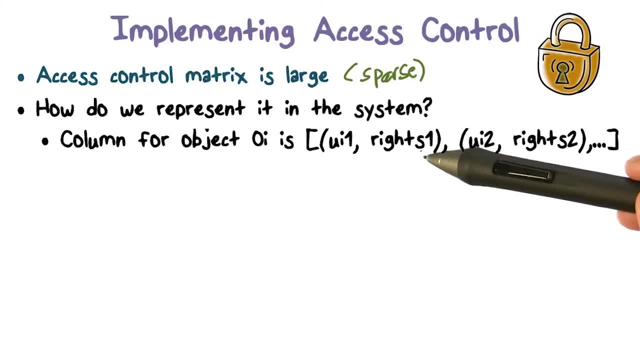 And we can sort of make a list that says: well, for object oi, user ui1, this user's access rights are this value: Okay. so this is sort of. we have these entries. So when I said matrices, when they're sparse, 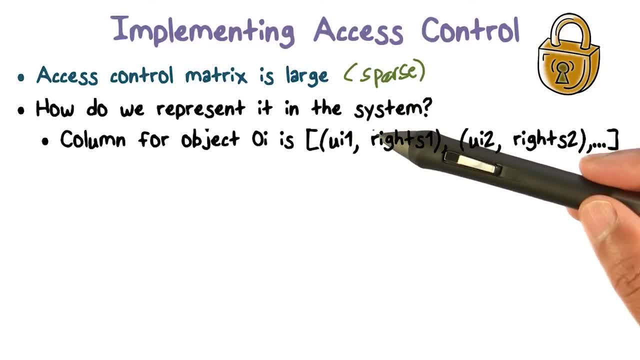 they can be implemented through link list, for example. So this could be a list of- and it's going to have a small number of entries, because most users don't have any access for object oi. So if a given user has access, what kind of access we can have? 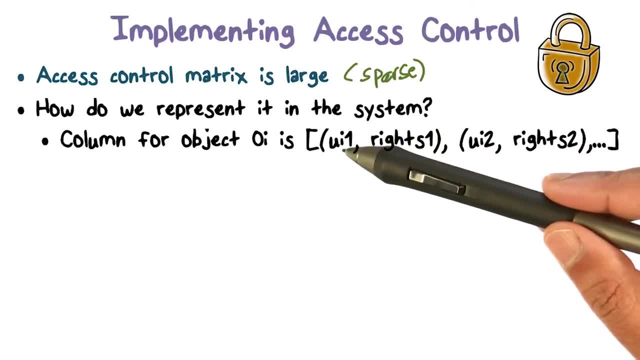 sort of this pair: the user ID and access rights. that makes up the first node in our list. The next user is going to be ui2, who has some other set of rights, and so on. So we can just sort of go down the column and 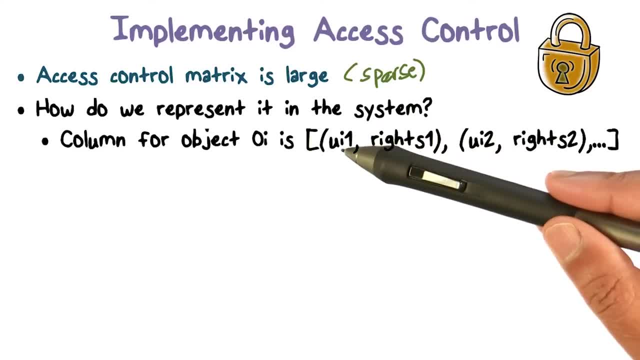 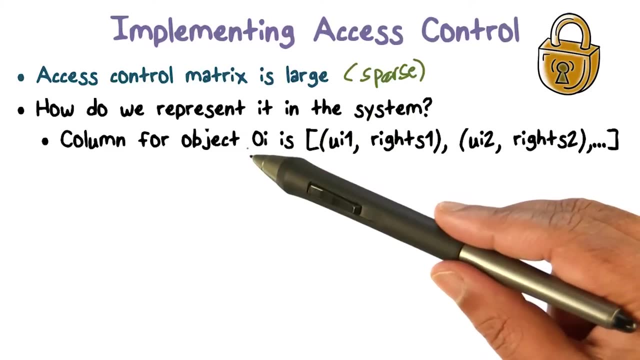 see what users actually have non-null access rights And sort of build these entries that become nodes in a link list or something like that, So we can organize this information Either by a resource or an object. Here we'll have to keep track of what users have access to this object and 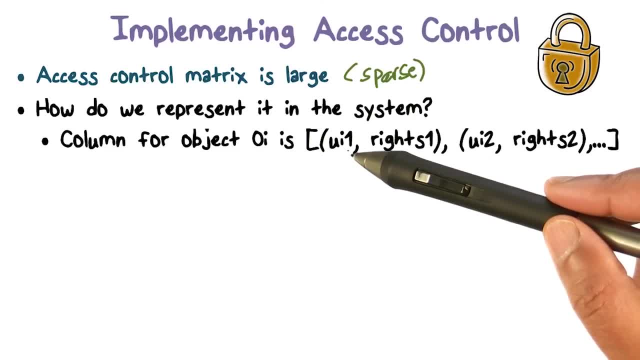 what kind of access they have for this object. So that's one way to do it. When you do that, this list I'm talking about, or the data structure that we're talking about, which is this collection, is link list kind of a data structure. 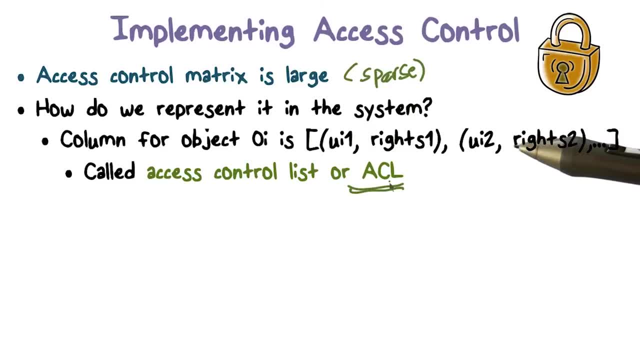 That's a collection of these entries- what user has what access rights. This is called an access control list or an ACL. So if you sort of focus on a resource or object oi And grab the information, who has access to this resource and 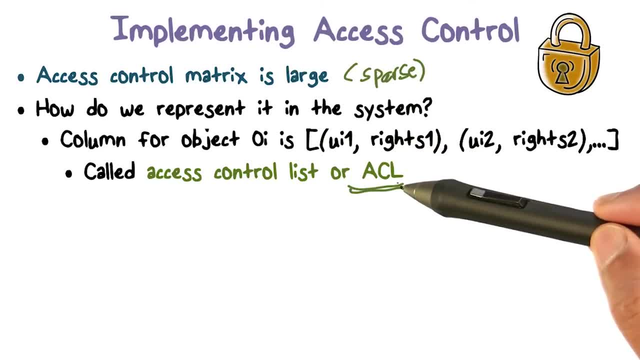 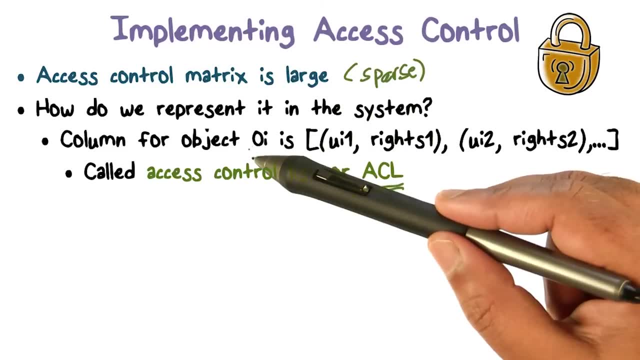 what kind of access. That defines an access control list or ACL. To keep in mind is that ACLs are for resources we have in the system, So ACL is always associated with an object or a resource. There's another way to sort of think about how we can implement it. 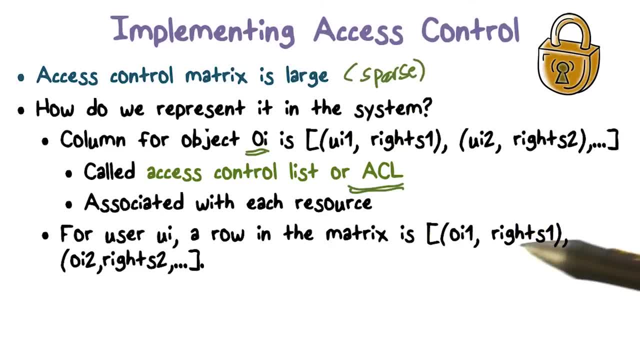 And rather than sort of focusing on columns, we can focus on rows, And we know that rows correspond to users. So we can go down horizontally, you know, across row, and say: so what would we see? If it's a sparse matrix, this user ui is not going to have access for.